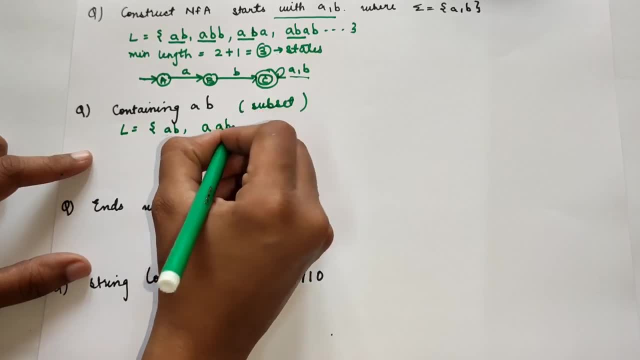 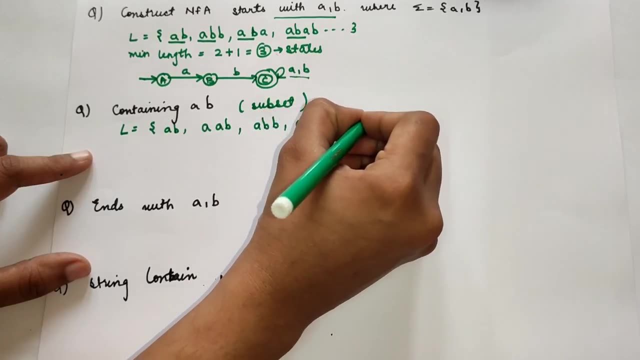 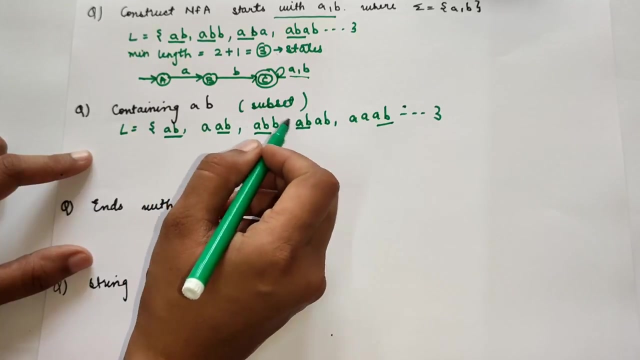 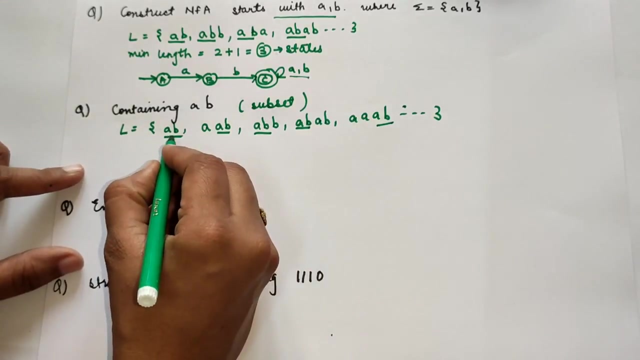 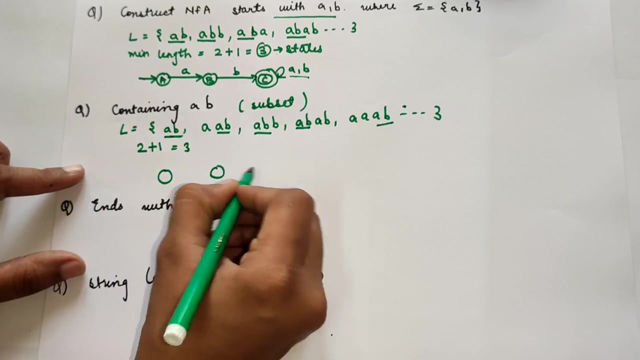 It can be AB, AAB. It can be ABB, It can be AB, AB It can be AA, AA It can be AB. It can be any combination, But it has to be a subset. There can be a subset, You have to remember. there has to be a subset of AB. It can be in the starting, It can be in between, It can be anywhere, It can be in between, It can be in the starting as well as it can be in the ending, But there has to be AB. So how we can draw? Obviously, the minimum length is 3.. Minimum length is 2.. What would be the possible states? Obviously, states would be 2 plus 1, that is, 3.. So draw 3 states. first Initial stage is this: 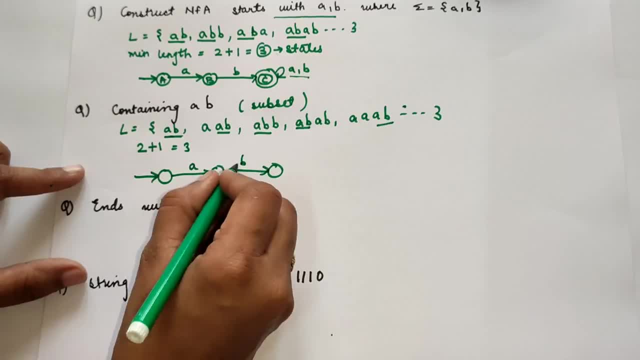 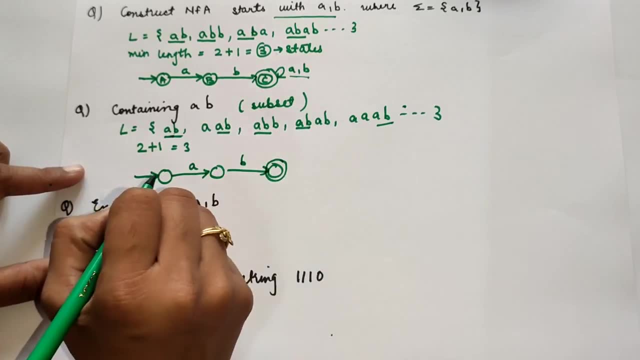 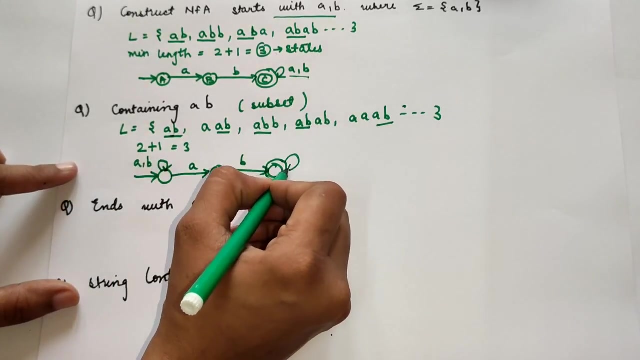 1 is the initial state And we have to accept it. The state We have drawn the NFA for this minimum length, That is AB. It is AB And obviously it is accepted. That's why it is a final stage Now. it has to be star. It has there can be, there has to be subset of AB. But before AB there can be any combination of A and B, So we can take closure of A and B here. Similarly, after AB there can be any possibilities of A and B, So we can also take closure of A and B here. So this is the minimum length. 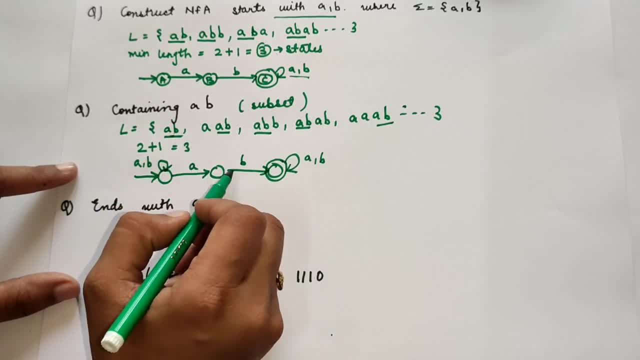 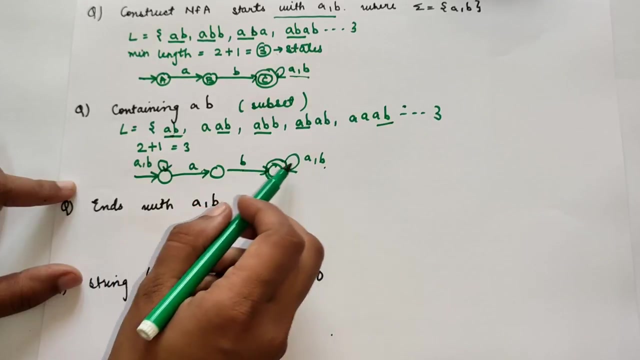 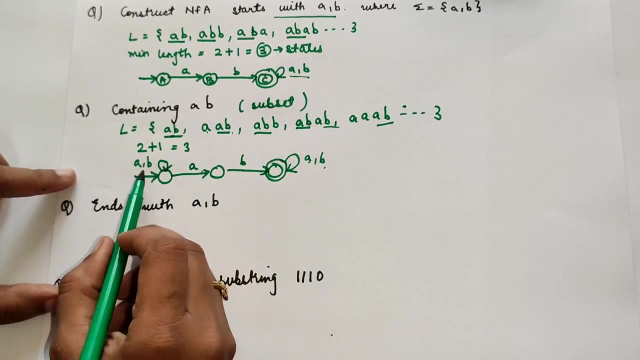 This is the subset for the subset of NFA. for this particular NFA, We can construct the NFA for this subset, AB, where there can be any combination of A and B, followed by AB, and there can be any combination of A and B. So you have to remember, even we can make it as null, It can be starts with A, B, then there can be A, So all the strings is going to be satisfied. You can check it Like, for example, A A B, Let's take A A B, Then we can take A, then A and then B, So it is accepted. 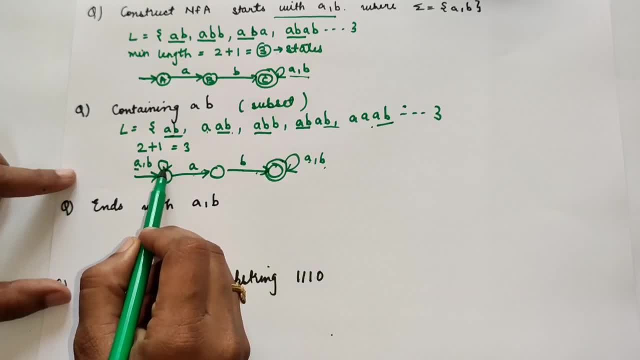 Let's take this triple A- B, Then first we can take A, second time A, then this third time A and this B. So this is also accepted. So in this way we can draw the NFA for containing A and B as a subset. 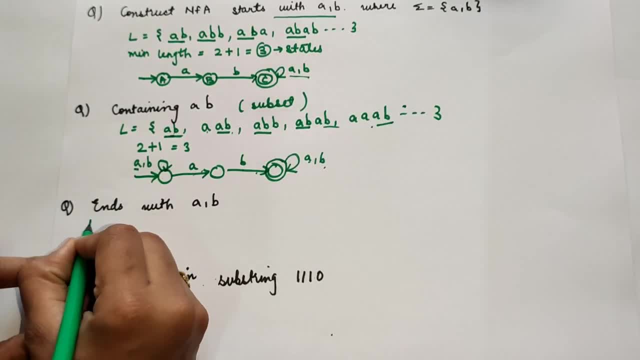 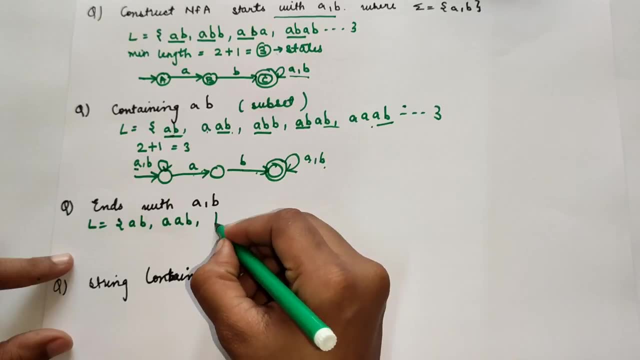 Now ends with A and B, Ends with A and B. again, language would be AB. It can be A A B. It can be B A B. It can be B, B, A B. It can be any combination, but it has to be any combination. 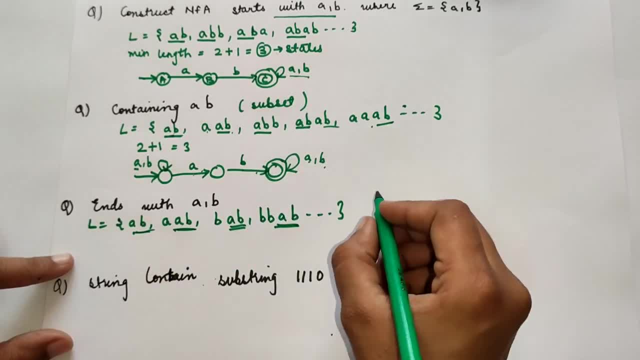 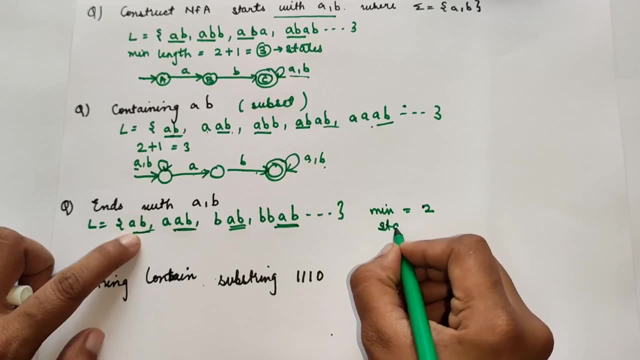 So it ends with A B. It has to be ends with A B. And again, what is the minimum length? Minimum length of substring is again 2.. And what would be the states here? It can be 2 plus 1.. It would possible states would be 3.. 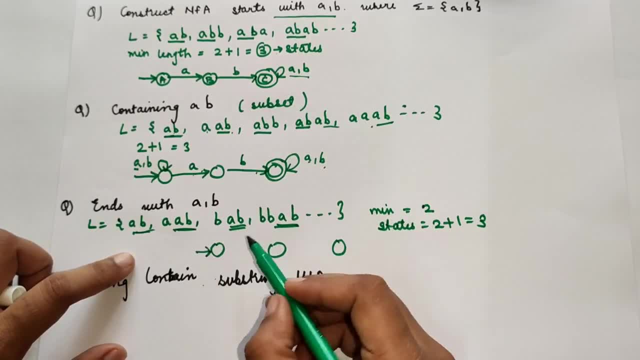 So first of all draw the 3 states, Mark the first stage as an initial stage. Then take the first string, that is AB. Minimum length is AB. So we have taken this string and obviously AB. It is also ending with AB, So it is also going to be accepted. 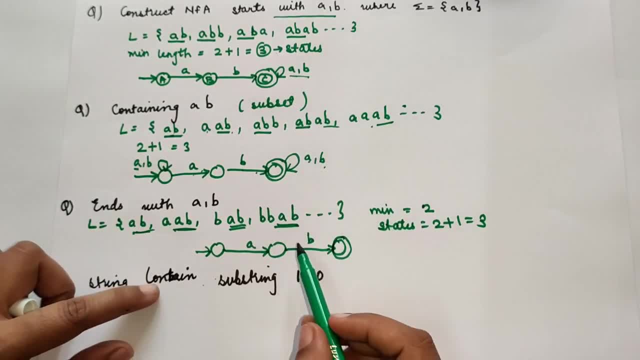 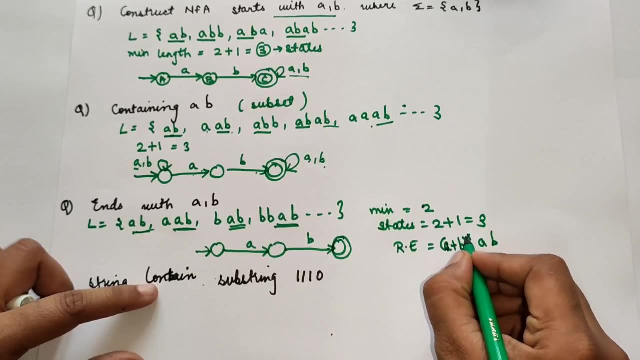 so mark it as in final stage. now see it has to be ends with nab. what would be the regular expression, it has to be ends with ab. but in starting can be: have any combination of a and b, so we can take closure of a and b. so in the first state we can take any combination of a and b so we can have a. 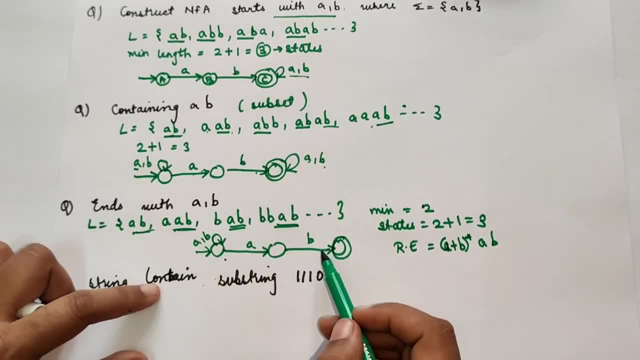 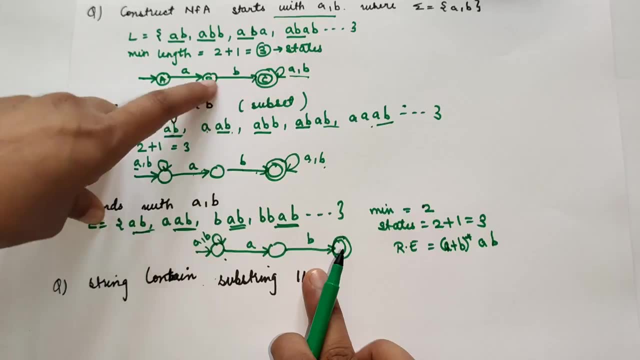 closure of this. so these are the possible. this would be the possible nfa. in this first one, you can see, the closure was at the end ab, followed by any combination, because here it is starting with a and b, but here it has to be ends with a and b. that's why we have taken closure at the first one. 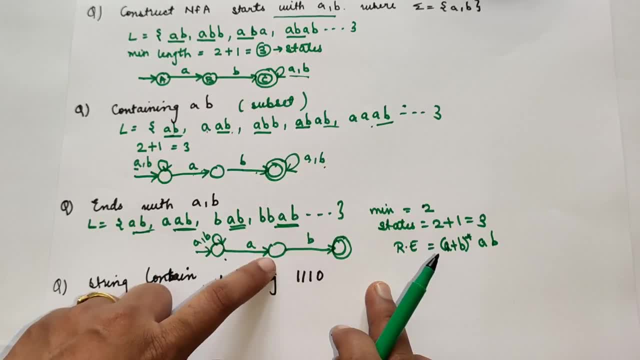 that is, we have taken the self loop for the input: a and b, then it is followed by ab, because it has to be end with a and b. let's take this example: bb, ab, whether it is accepted or not- b, again b, then a and b. it is accepted because it is reaching to the final state means it is a correct nfa for. 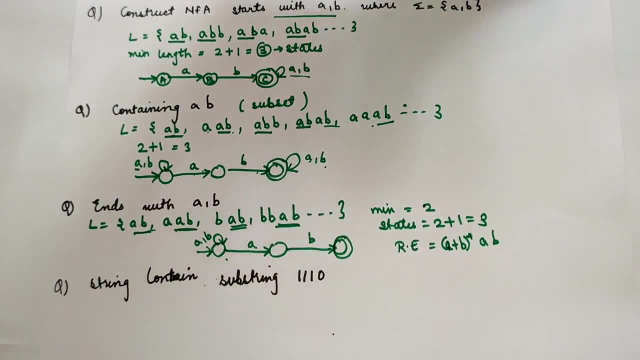 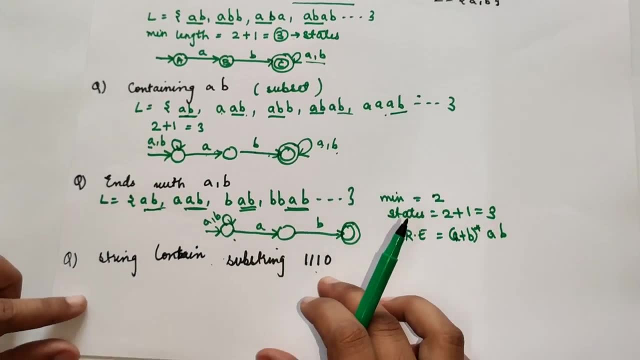 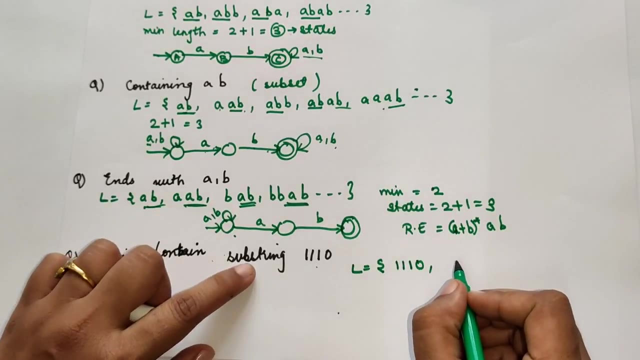 the given input. now we will take one more example. for the string containing substring 1110, triple 10, what would be the possible nfa for this? we will try to draw, see. first of all, we will try to write down the language. what would be the possible language? 110 can be. it has to. they have mentioned. 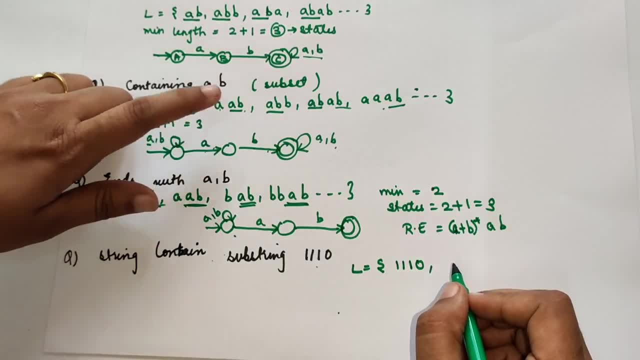 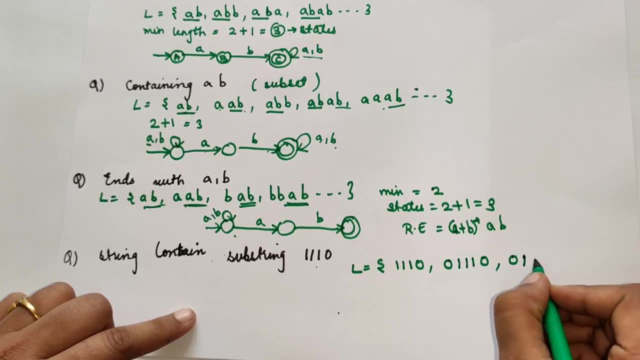 it has to be substring. it is very similar to this one. it is similar to containing a and b. it can be 0, triple 10. it can be 0, 1, 1, 1, 0. it can be triple 1, 0, 1. it can be this one. so you can see. 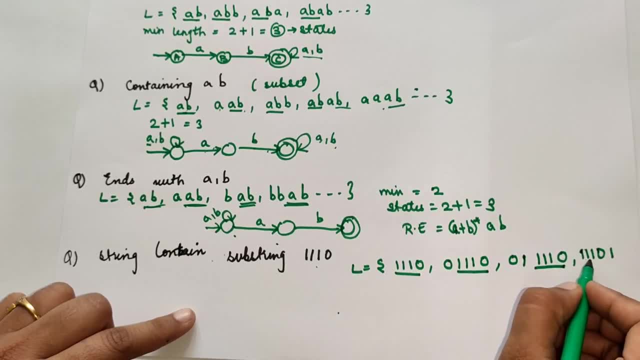 i have written. every time i have written the subset as a triple 1: 0. after that there can be one, there can be previously, there can be 0 and then at the last there can be anything. so it can be have any, any combination of this, but the subset has to be triple 1: 0. so minimum length is again: you can see 1, 2, 3 and 4. so first, 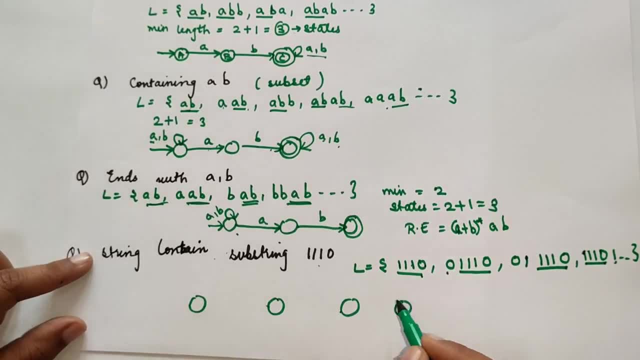 of all, we'll draw four states: 1, 2, 3 and 4. there are, these are the four states. obviously, first state would be the initial stage. now we'll try to write down the input first. we'll write down the input is that 1, 1, 1, c, this has the minimum length of a string. minimum length is 1, 2, 3 and 4. so states: 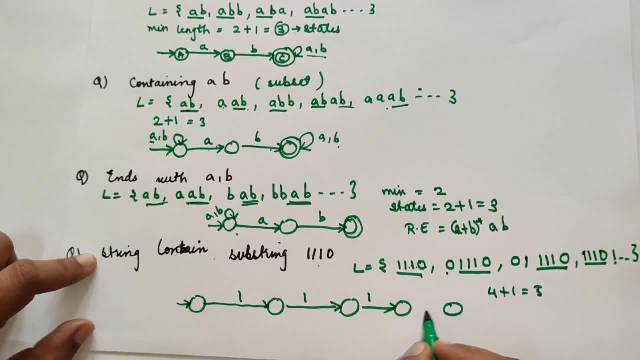 calculated using 4 plus 1, that is 5 states. so one more state would be there, that is 0. okay, so this would be the states here, and obviously 1 1 1 0 is going to be accepted, so we can mark it as a final. 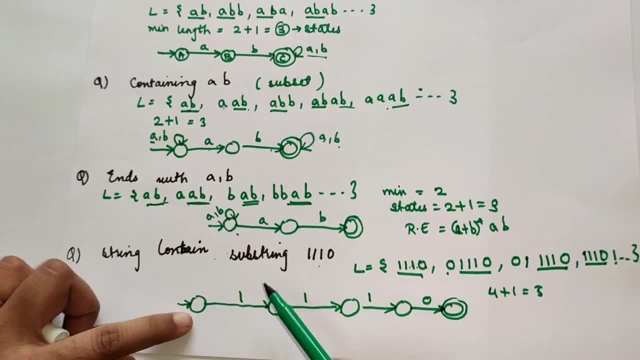 stage. okay. so now we'll try to make the another changes before. see in this subset. before that there can be 0, even there can be 1, so we can say that we can say we can take a self loop for zero and one, we can take a closure for 0 and one in even after triple 1, 0, it will come 1, 0 there can. 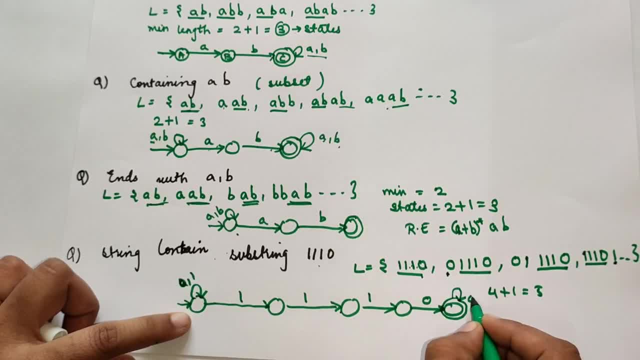 be any condition. there can be one or there can be 0. even for this we can take a closure of 0 and 1. so let's check. let's check for 0, 0, triple 1, 0, 1. okay for this combination, whether it is accepted. 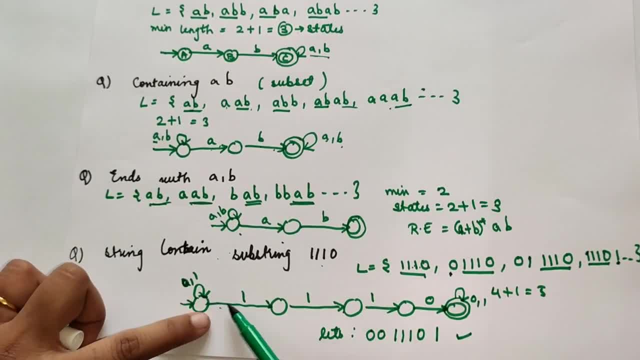 or not. let's check 0, again 0, then 1, 1, 1. I have forgotten. yes, it is 1, then it is 0, then, lastly, again, it is 1. so it is accepted because it is reaching to the final state. so this would be the. 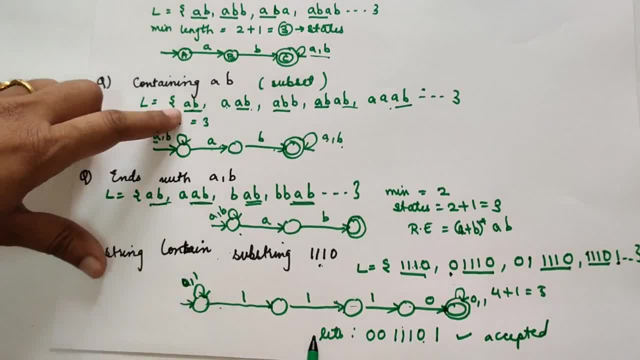 possible NFA for the substring. this one similar, it is very similar to this. you can see, at the starting there was AB, at the ending was also there was AB. here also there is starting at 0, 1, closure of 0, 1, and here it is also closure of 0, 1 and in between there has to be substring ripple 1, 0. so 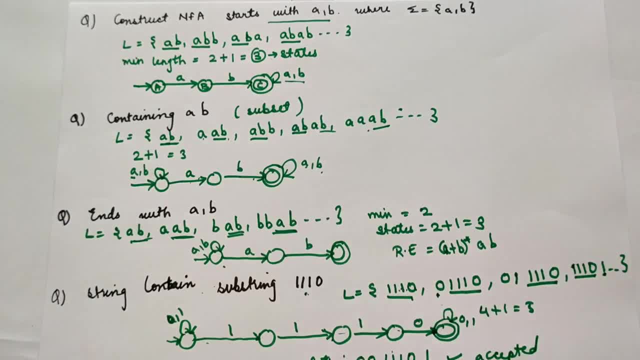 in this way we can draw the various NFA. we'll see some more examples in our upcoming video.